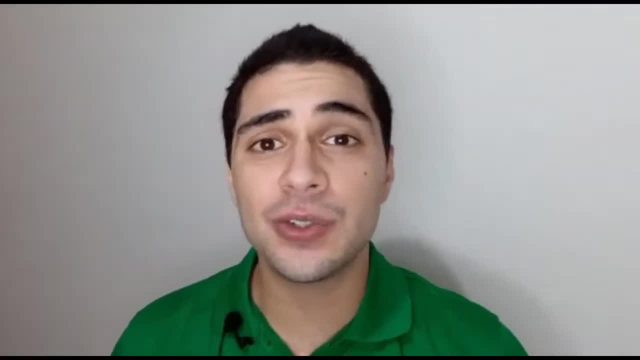 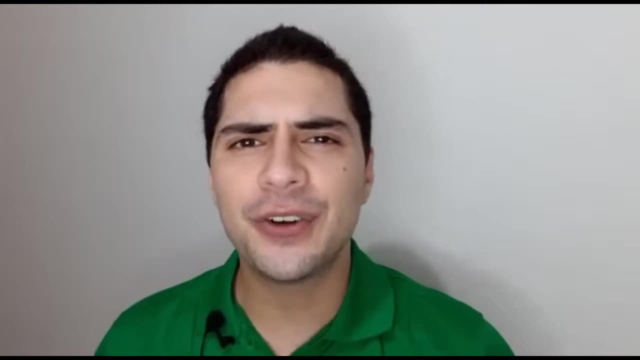 Oh my god guys, welcome to another video. today's video tutorial is going to be very, very helpful, but before we continue with the video, guys, it's very helpful to me and for the oh my god community to grow for you to hit that subscribe button and that notification bell if you find this. 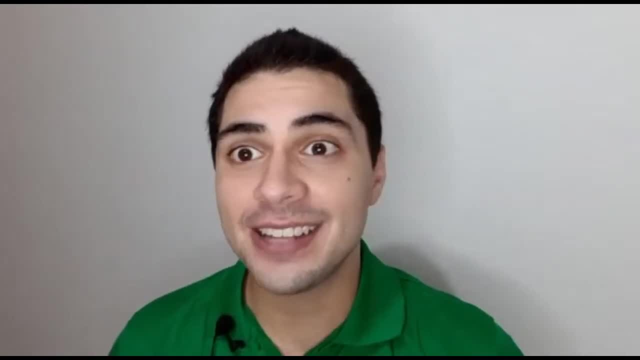 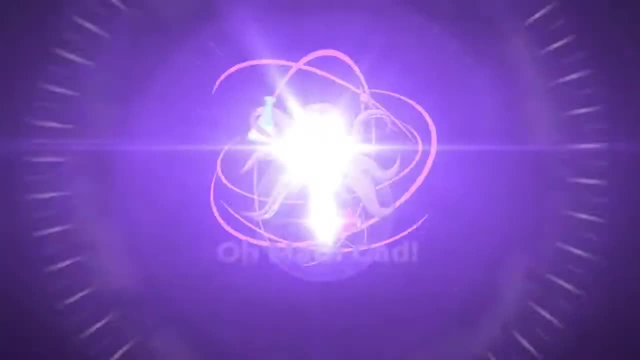 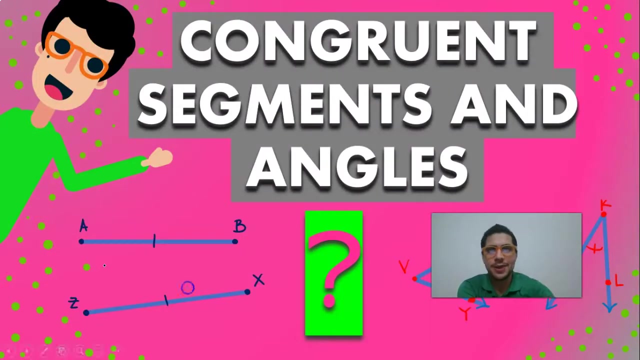 video useful. don't forget to leave a like, a comment and again subscribe. let's begin. oh my god. okay, welcome back everyone. hope you guys are doing amazing. today's video is about understanding congruent segments and angles, what they are used for, how we can recognize them. 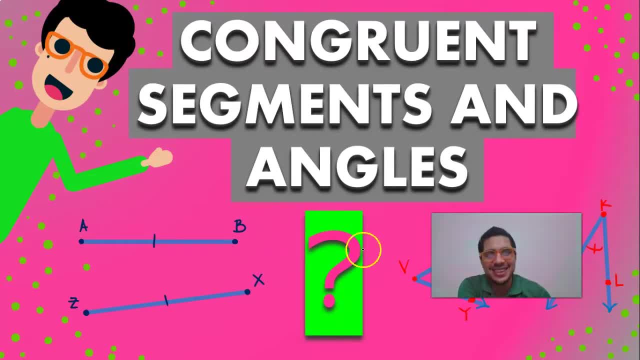 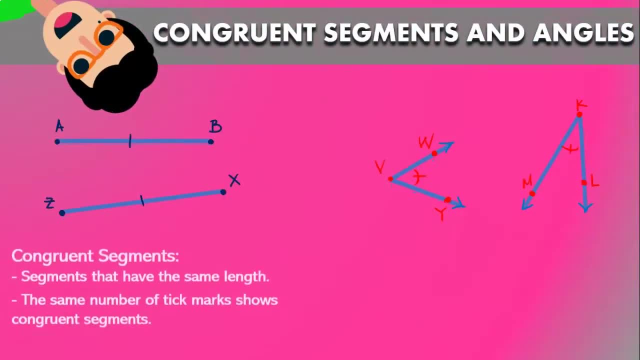 and how can we actually use them in a problem. so let's begin. so we're going to be learning about congruent segments and angles. first of all, congruent segments are segments that have the same length and the same number of tick marks shows that the congruence um the segments are congruent. so in this, 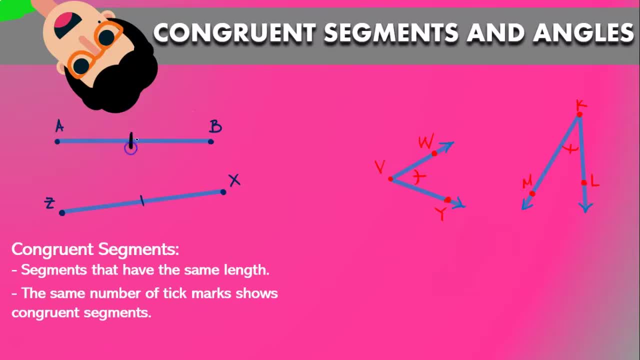 case, we have a- b, we have a single tick mark and we have z x and we have also a single tick mark. that means that a- b is congruent and this is the symbol for congruent with z x. okay, so that means that whatever is the length of the segment a- b, the length of a- b is going to be equal to the length of. 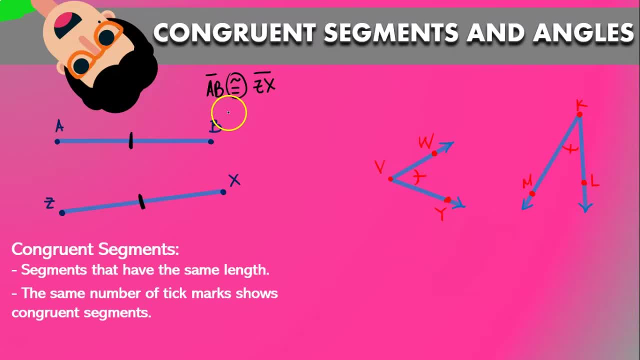 z x. so if a, b is five centimeters long, z x is also five centimeters long, and we're also going to be talking about congruent angles. so the same thing. Concurrent angles are angles that have the same measure and the same number of tick marks or arc. 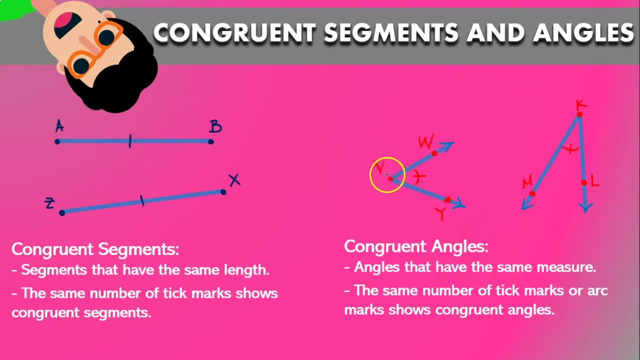 mark shows that actually two angles are congruent. So in this case, the measurement of the angle WBY, so WBY- is going to be the same as the measurement of the angle MQL or LQM, So LQM. Why? Because, since we have the same tick marks and the same arc marks, we know that the angles 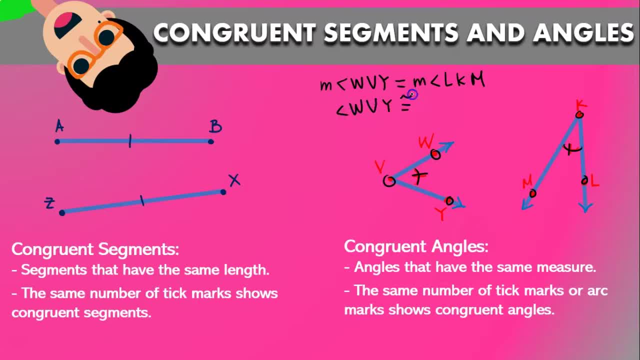 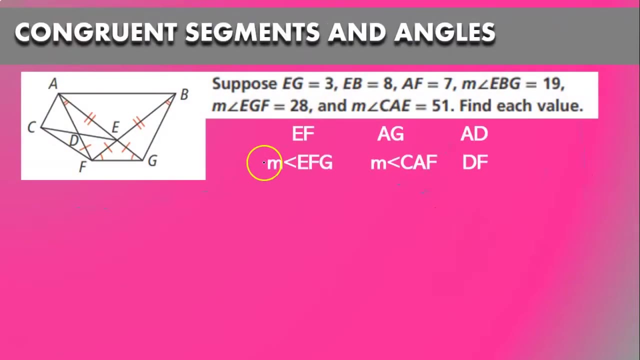 are congruent, And if two angles are congruent, that means that their measurements are equal. Okay, so we have to take that into account. Now we're going to try solving a problem. So suppose EG is equal to 3, EB is equal to 8, AF is 7.. 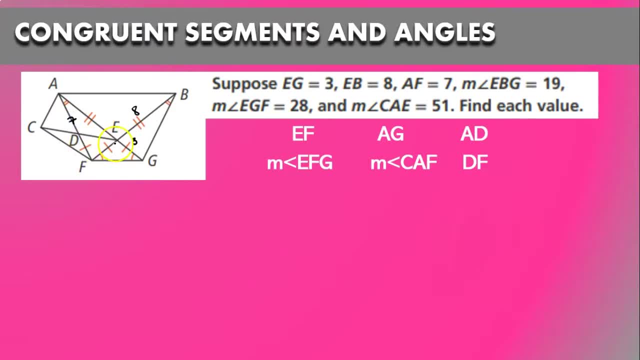 The measurement of the angle WBY is equal to 8.. The measurement of angle EBG- EBG- so this one right here- is 19 degrees. The measurement of angle EGF- EGF- so this one right here is 28 degrees. 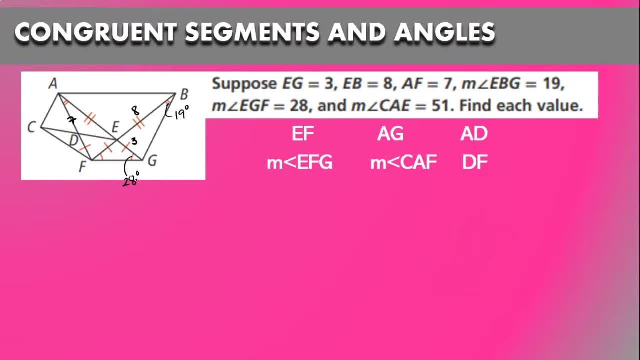 And the measurement of angle CAE, again CAE. so this whole angle right here, CAE, And the measurement of angle CAE is going to be 51 degrees. So find each value. So the first value they're asking us is EF. 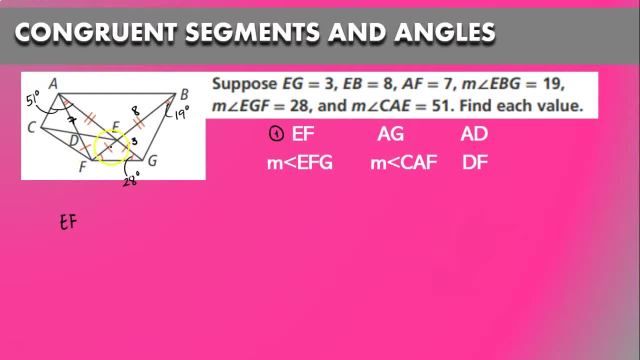 So, as we can see, EF has a single tick mark and that single tick mark is shared with EG. That means that segment EF is congruent with segment EG. That means that EF is equal to the measurement of EG, so EF is equal to 3.. 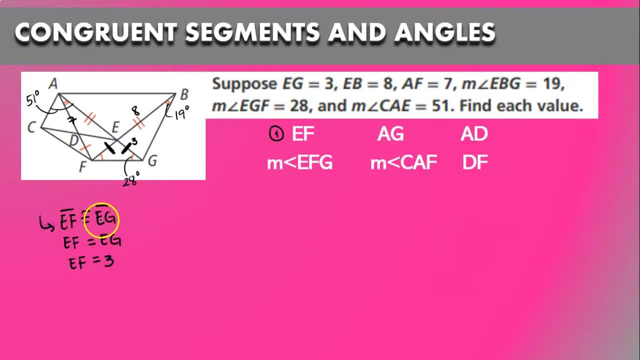 It is very important to first say that it is congruent and then I can say that the measurements are equal. If I skip a step, be mindful, because you may be losing points right there in the procedure. Thank you. Next we have AG. 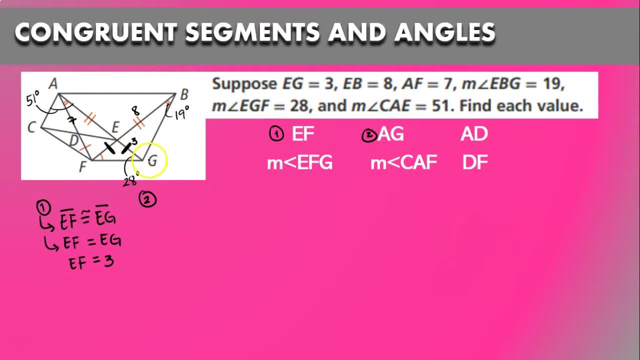 So again we have AG. AG is the same thing as AE plus EG, correct? And now AE has the same tick mark as EB. So we know that AE is congruent with EB because they have the same tick mark. So AE. 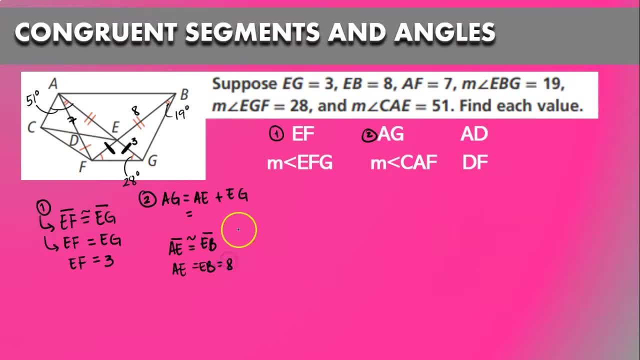 is equal to EB. that means that it is equal to 8. so AE is 8 and EG is 3. so 8 plus 3 is 11. now we go with 3, which is a D, now a D. a D is going to be the same as a F, which. 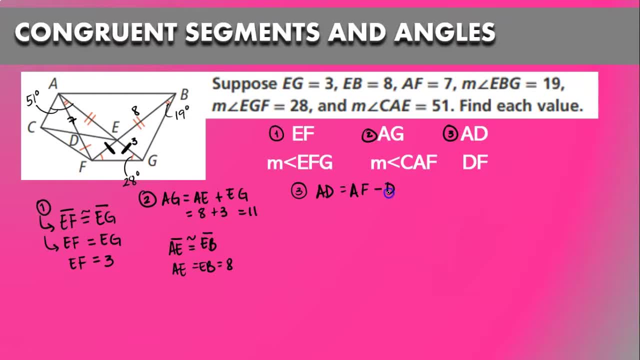 is the whole segment minus D F. we know that AF is 7 and we know that D F is actually just going to be 3, meaning that ad is going to be 4. what about EF G? okay, okay, so e f g has the same mark as e g f. that means that they are going to be congruent. 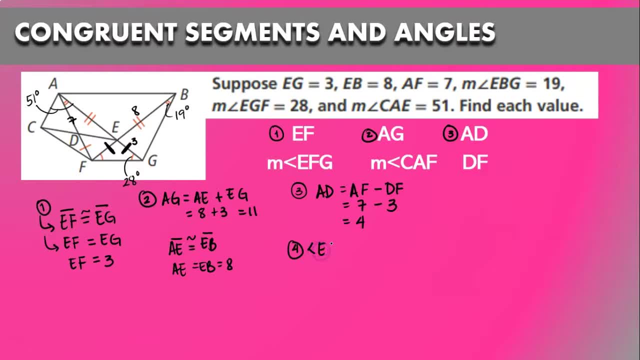 so the angle e f g is going to be congruent with angle e g f, meaning that their measurements are going to be equal, and what that means is that it's going to be 28 degrees. what about c a f? well, c a f is going to be just this tiny bit right here. 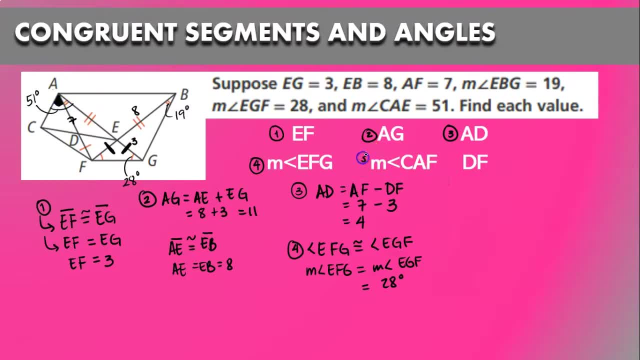 and the measurement of angle c a f is going to be the measurement of angle c a e, minus the measurement of the angle f a e, and because we know that the angle f a e is the same as the angle e, b, g, that means that that is going to be 19 degrees. 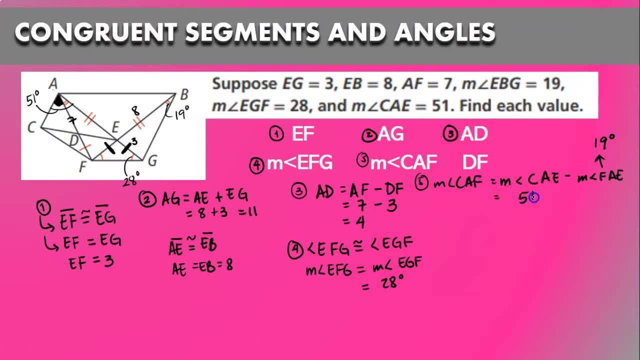 so that means that c, a, e, which is 51 degrees, we're going to subtract, we're going to subtract 19 degrees. so that means that the angle is going to be 51 minus 19 degrees, which is going to be 32 degrees. and then, last but not least, we have d, f and d? f, we have the same. 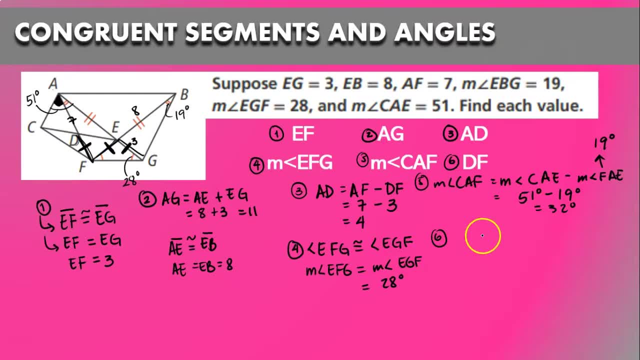 tick mark as e f and as e g. so d f, the segment, is going to be congruent with e g. so that means that the measurement of d f is going to be the same measurement as e g, which is going to be three, and that is going to be your and, as you can see by this procedure right here, it is not as 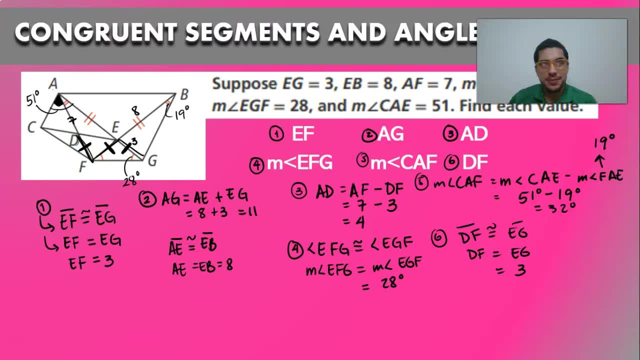 complicated. you just have to remember quite some things. as you can see, in this problem of congruency you have to actually use problems of the postulates we have already seen and you actually have to remember to first put the two segments or two angles are congruent in order. 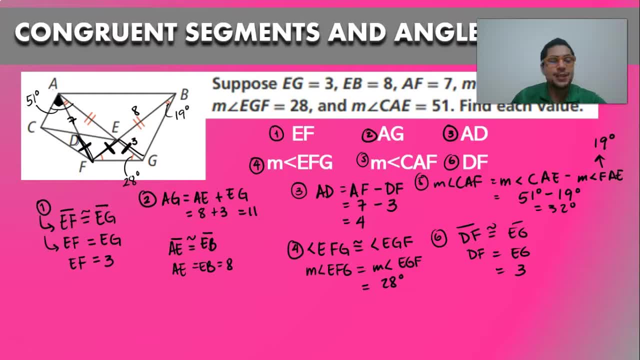 to say that their measurements are the same, and that's pretty much it, guys. so i would recommend you um starting from scratch and then doing it once or twice more, so that you get those math skills boosted, and i'll see you on the next one. bye, bye. 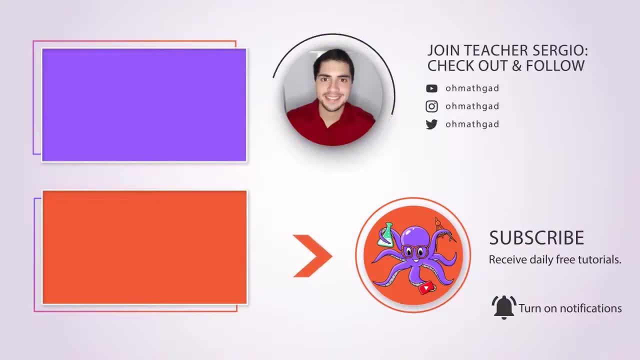 guys, check out these other videos to improve your math skills and make sure you click that subscribe button to make the community grow. follow omath god in its social media accounts. drop a like a comment below and see you on the next one. bye. 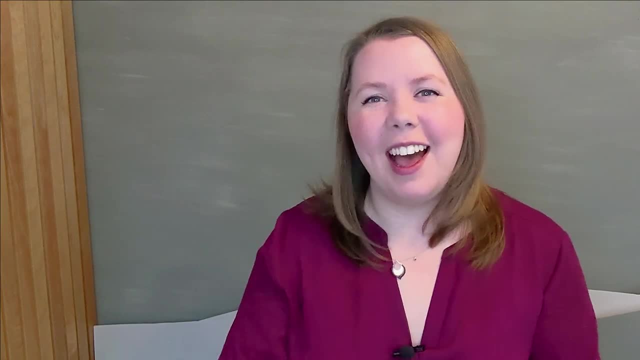 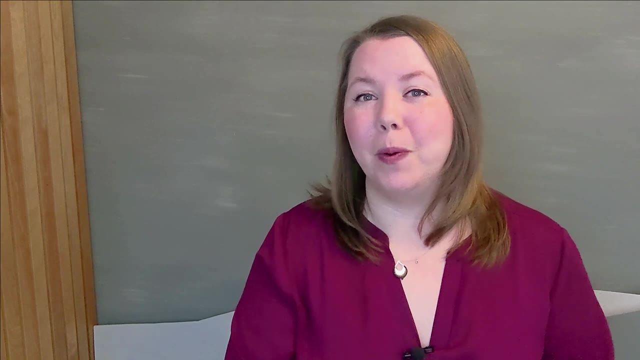 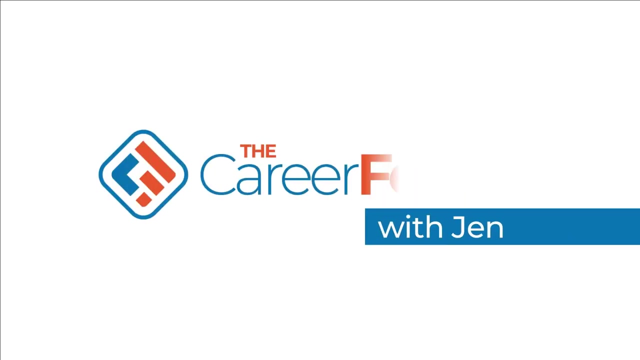 What does a healthcare data analyst do on a daily basis? Hi, I'm Jen and I've worked in analytics for 15 years. Now I work as an analytics consultant and help other people break into analytics roles. Let's get into what a healthcare data analyst does. Here's what you can expect in. the day-to-day role of a healthcare data analyst. Like almost every data analyst role, the answer to what does a healthcare data analyst do isn't just one single answer. There are many niches within this broader category of healthcare data analyst. There are certainly similarities across.